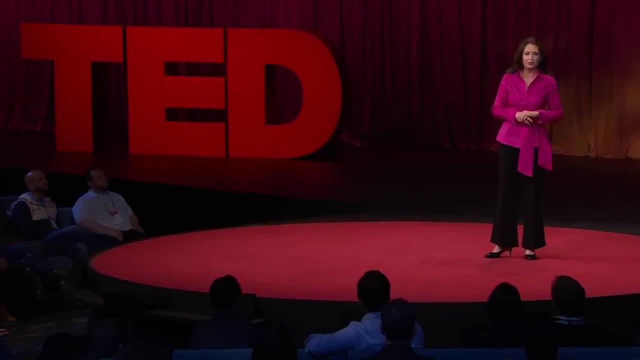 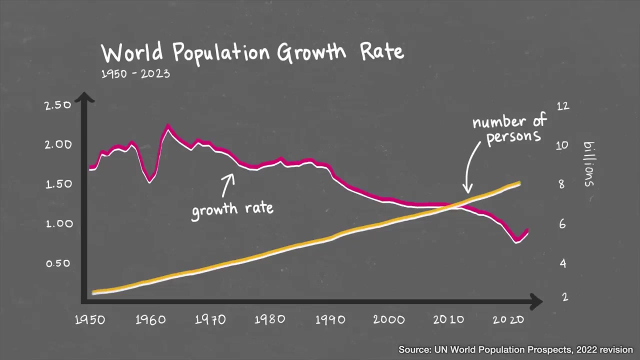 which is obvious, total growth and the tectonic forces beneath. Since the 1960s, world population has more than doubled, but the growth rate has been falling the entire time. We're witnessing the most fundamental shift to take place in modern human history. 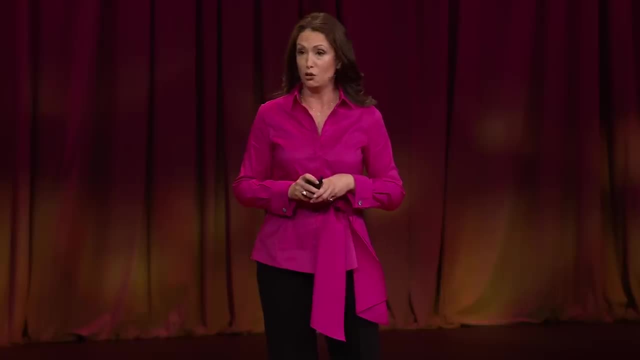 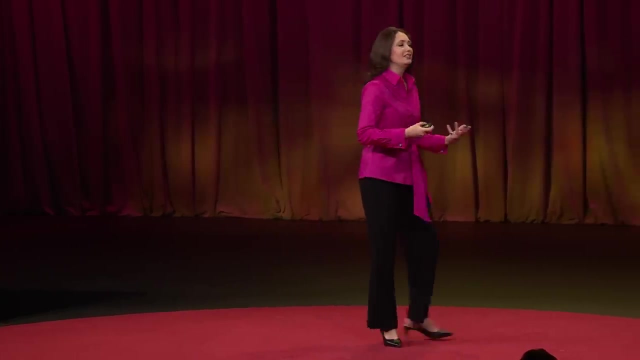 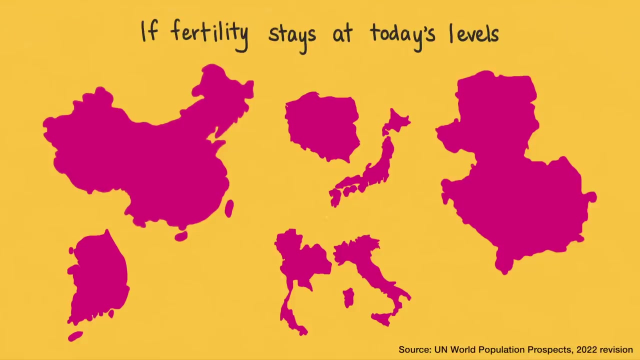 the shift towards pervasive and permanent low fertility, population aging and eventual depopulation. Fertility is down everywhere, just at different rates in different places. If fertility stays the same as it is today, just hold still by the end of this century. 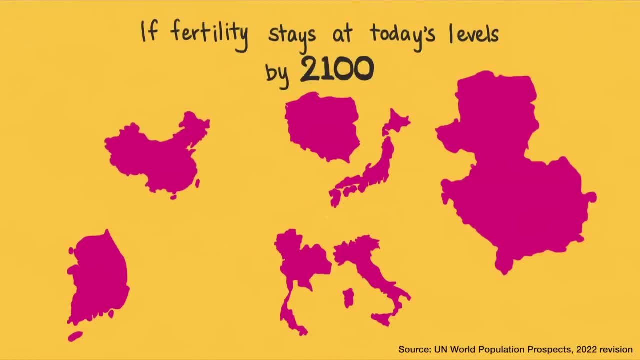 China's population will be less than half of its current size. It's a loss of 800 million people. South Korea's will be down by 63 percent, Poland's and Japan's by half, Italy's and Thailand's by 44 percent. 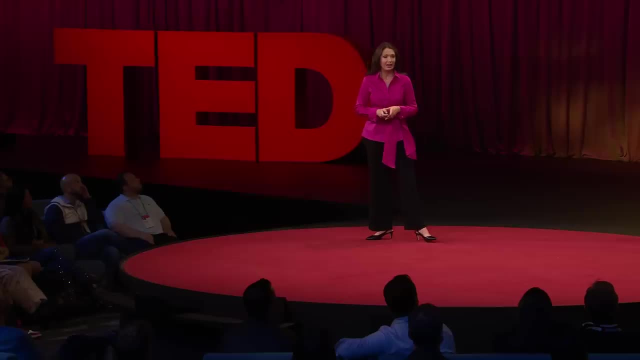 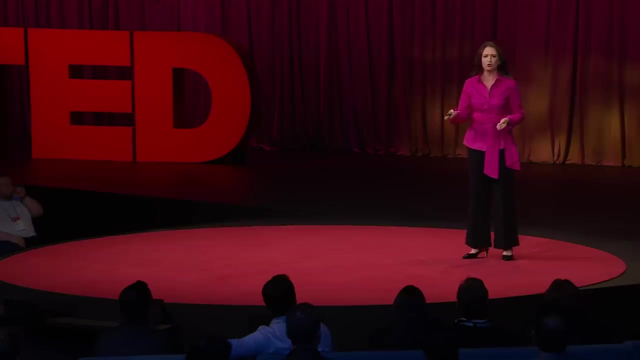 Eastern Europe by 40 percent. Even greater number of countries are already aging Again. just 20 years ago, if we'd lined up everyone in Japan or Italy or Germany, from the youngest person to the oldest, and we asked that person who wasn't in the middle of their age, 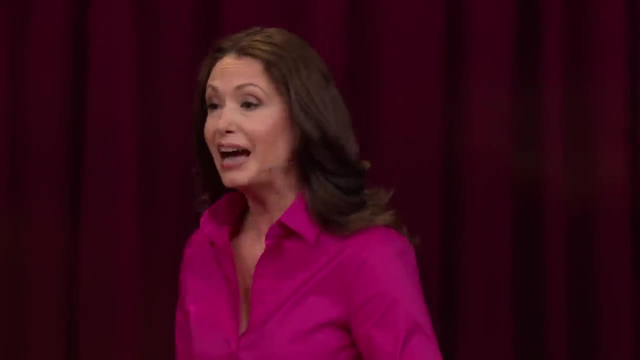 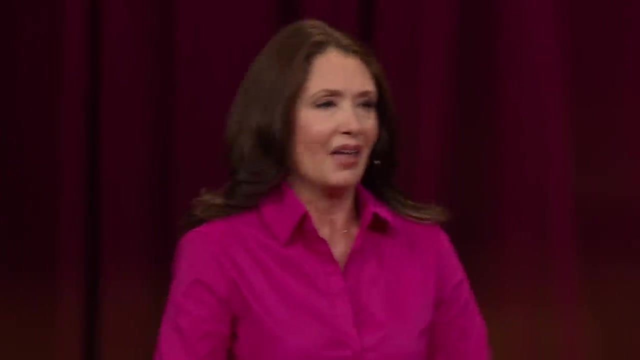 they would have been 40 years old. Today, the populations of Thailand, Kuwait and Cuba are just as old, with Chile, Iran and Vietnam close behind, And even India, as it seems to be this bright star assuming the throne as the world's most populous country. 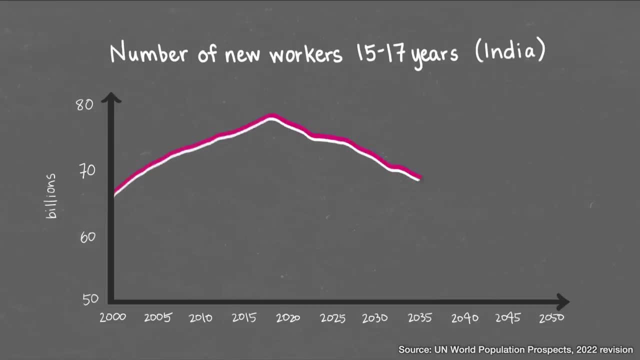 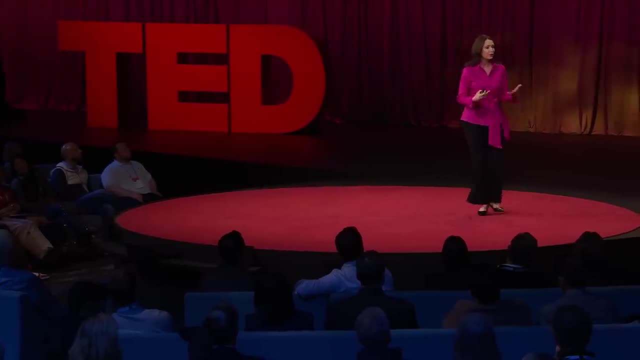 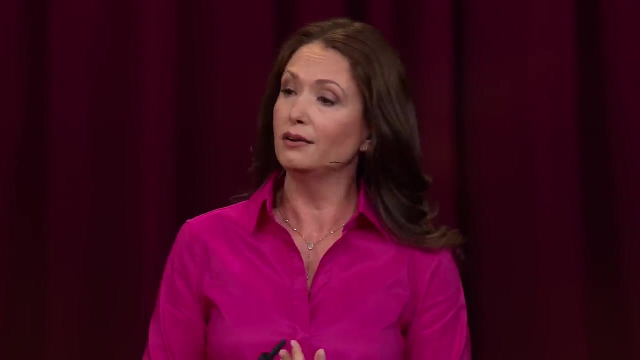 has below-replacement fertility. The number of young people entering into India's workforce has already peaked. People are the foundation of everything in a society. We're the workers and the voters, and the soldiers and the caregivers. So how many of us there are and who we are that matters. 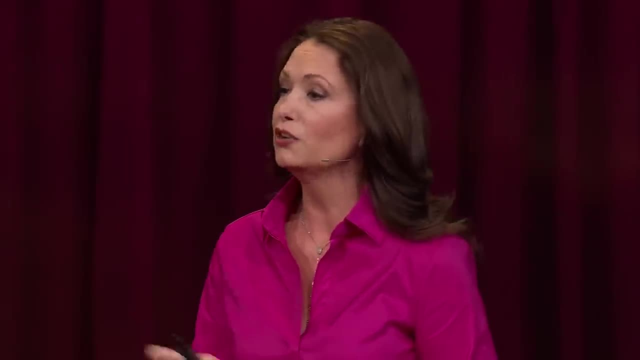 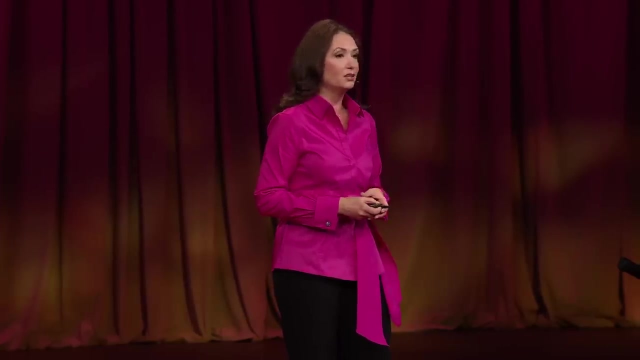 We're on track for there to be more people over age 60 than under the age of 14 by the middle of this century. That radical shift in modern human society presents us with a world of possibilities. Our demography is our destiny. yes, 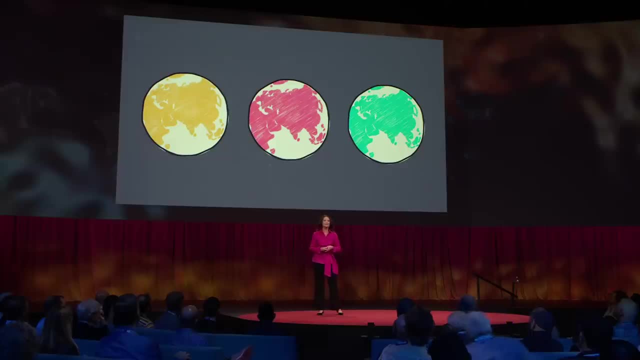 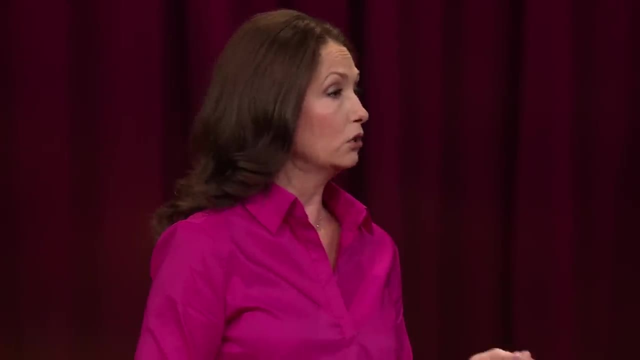 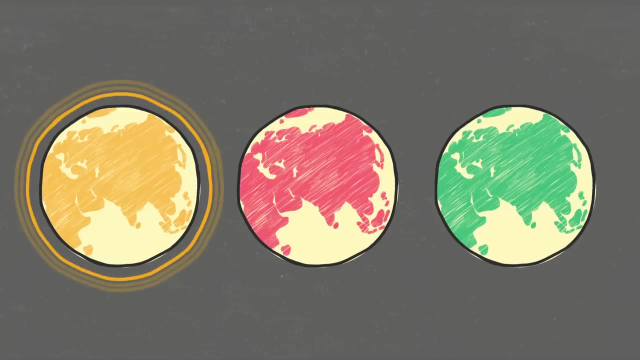 but how we react to that. demography is not preordained. What possible worlds might we create if we thoughtfully plan for an older, smaller population? In one possible world? we put our heads in the sand and keep going about our business as usual. 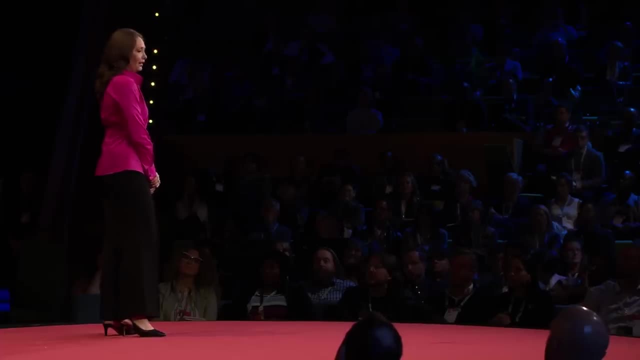 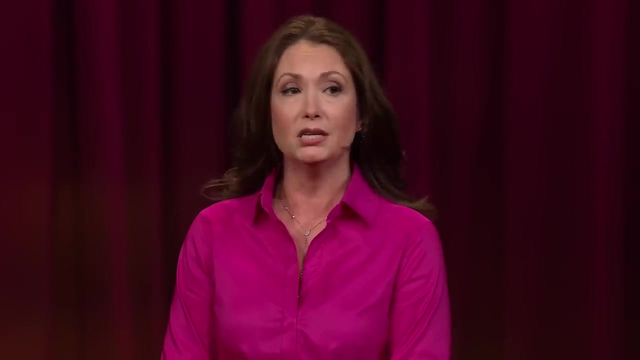 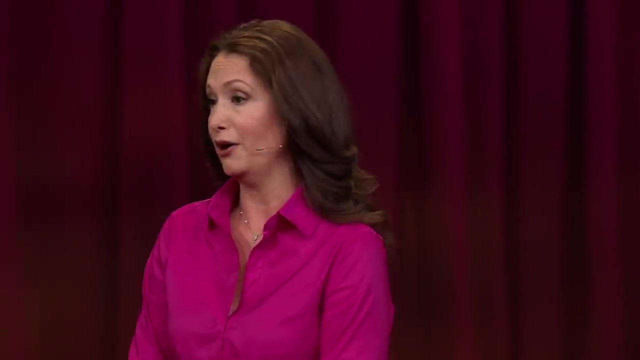 We have seen most societies react like they're living in this world and throw money at people to have more babies, but it doesn't work. South Korea has spent $210 billion over the last 16 years trying to raise fertility and they keep hitting record lows: under one child per woman on average. 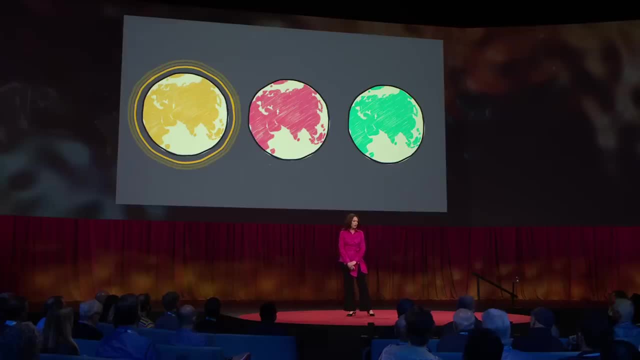 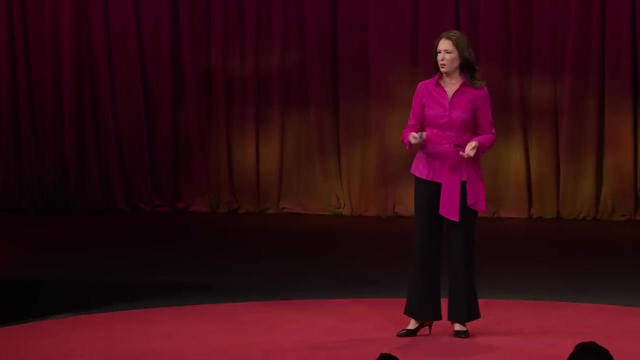 In this status quo world, we keep the same economic models that assume infinite population growth and amass more debt to pay for our public spending. Our social safety nets stay the same, which those rely on more inputs from workers than withdrawals from retirees. That's what we call a pay-as-you-go system. 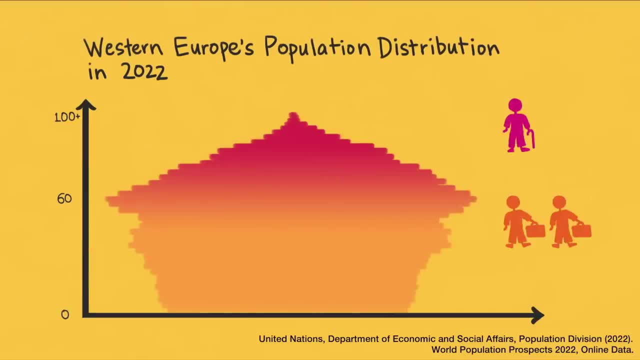 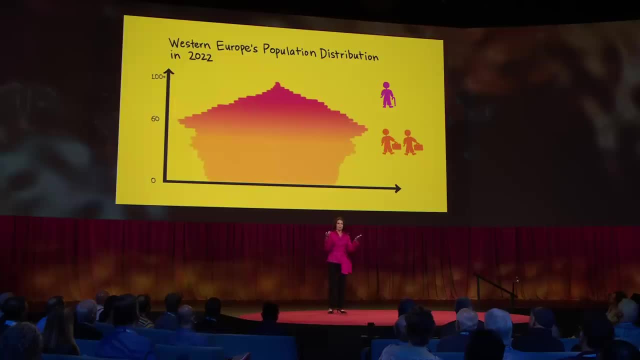 Western Europe is already struggling to keep these systems afloat, because in many of those countries there are only two workers for every retiree. You can see how top-heavy the population's age structure is here and how in the next few years it will grow even more so that way. 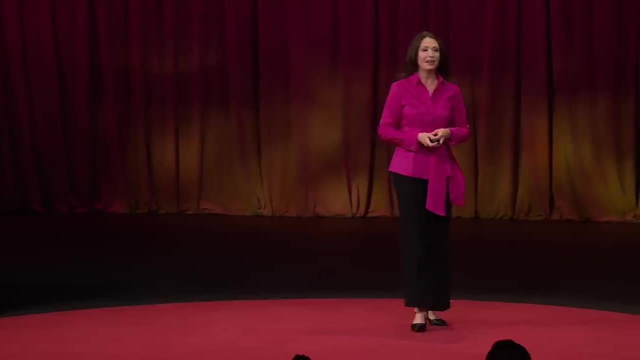 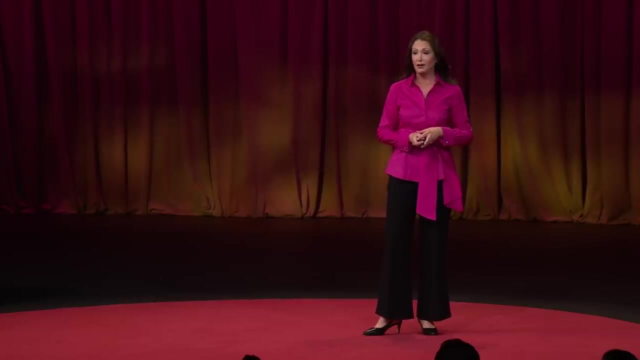 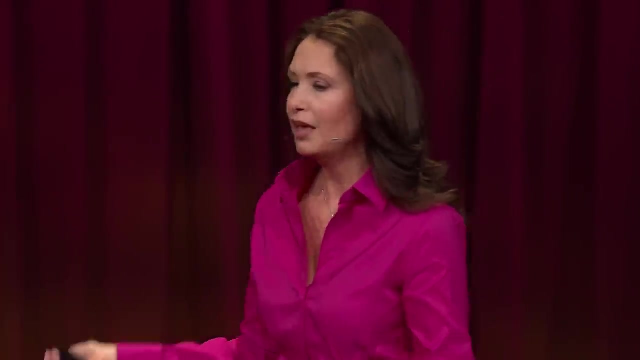 In a status quo world. the world's most powerful countries continue to increase military spending and try to project power beyond their borders, even as their national budgets strain and the recruiting pool for soldiers shrinks. Hello Russia, China and maybe even the United States. So what results from failing to adapt and clinging to the status quo? Well, systems overload and break. We have higher labor costs, which lead to inflation, and that just makes it even more expensive to have children. Social security systems go bankrupt and we lose the gains we've made in reducing old-age poverty. 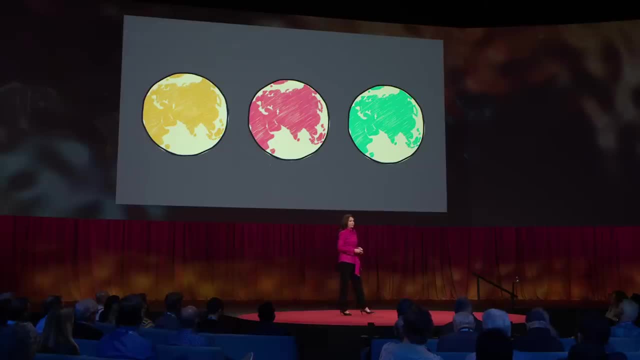 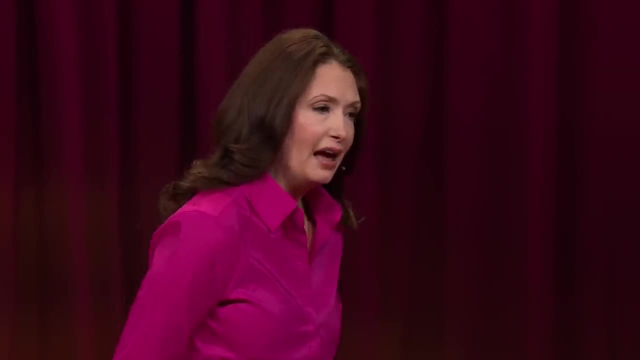 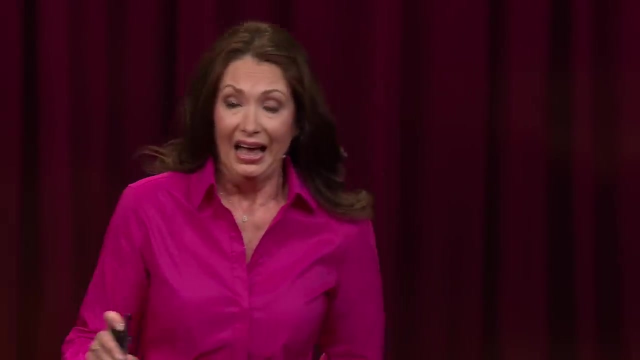 But a head-in-the-sand world isn't as bad as a fearful one. In a fearful world, the ability to choose how many children to have and when to have them gets taken away, something that's easier in less democratic settings, And not good news here either. 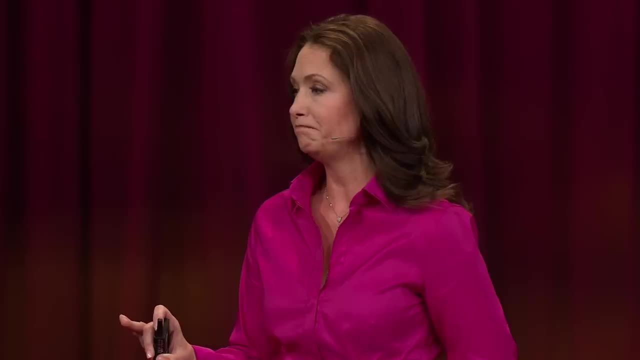 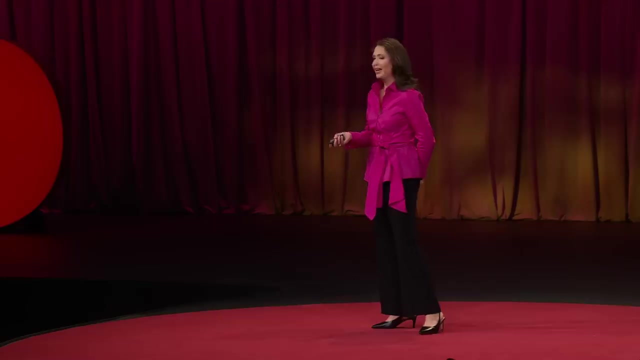 Twenty years ago, almost all of our aging countries were democracies. Now a quarter of them, those with median ages of 35 or higher- aren't free, And I know we see this idea of coercion in science fiction. but it's not just science fiction. 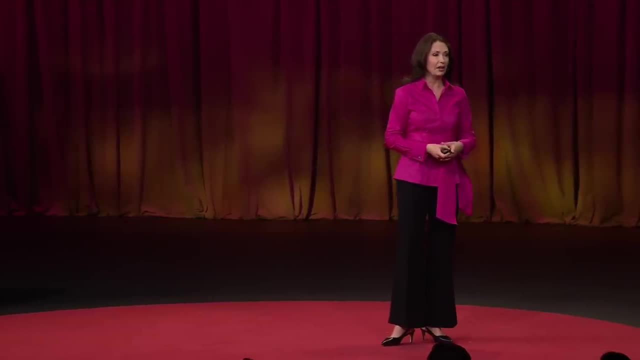 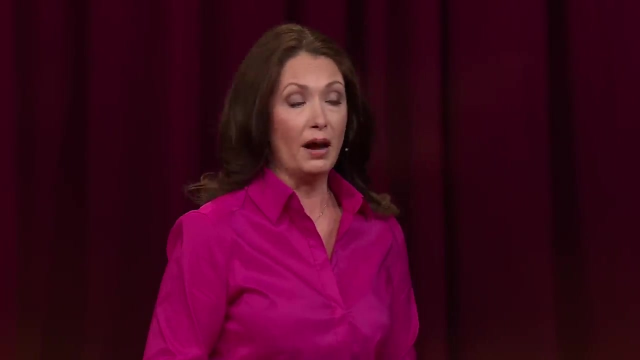 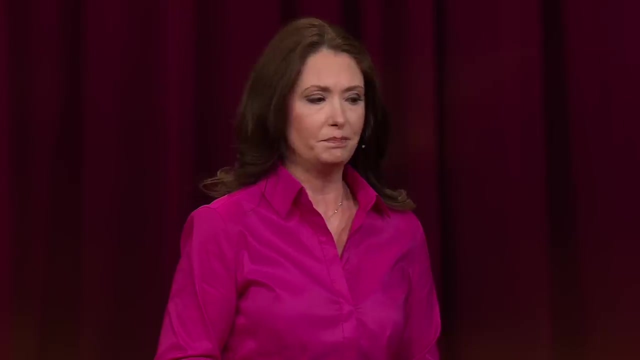 In 1965, when Nicolae Ceausescu took the helm in Romania and he wanted more Romanian babies, he forced it to happen through invasive measures. Fertility temporarily spiked, but not without dire consequences for women and for those children, many of whom were abandoned to orphanages. In a fearful world. immigration becomes more restricted. There's more hatred and division, as majority groups fear being replaced by people who don't look like them. There's less global cooperation as aging, shrinking countries lose the willingness and ability to think about causes outside their borders and fund those. 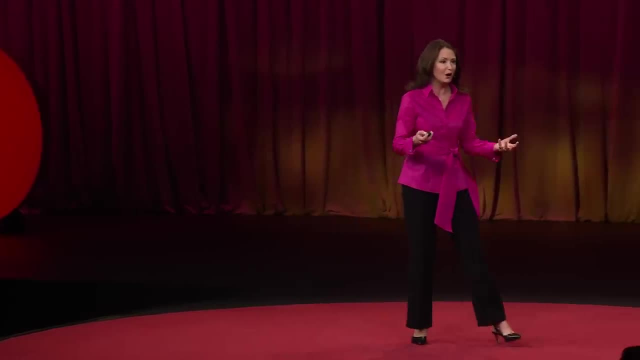 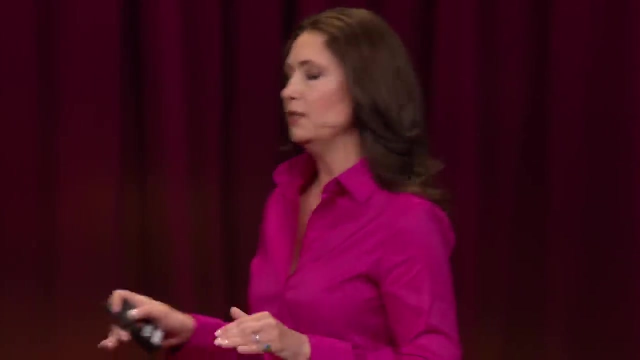 We can't come together on pandemics or climate change or other transboundary issues. Does any of this sound familiar? I actually don't think we're fully in this world yet, even if way too much of this hits close to home, But I can imagine how we might get there. 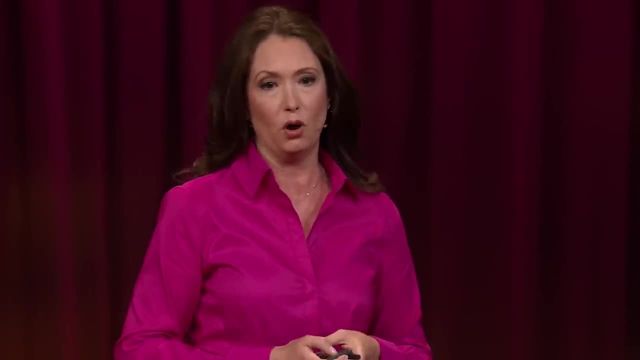 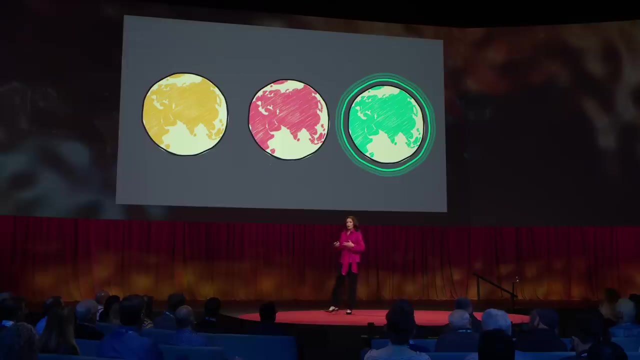 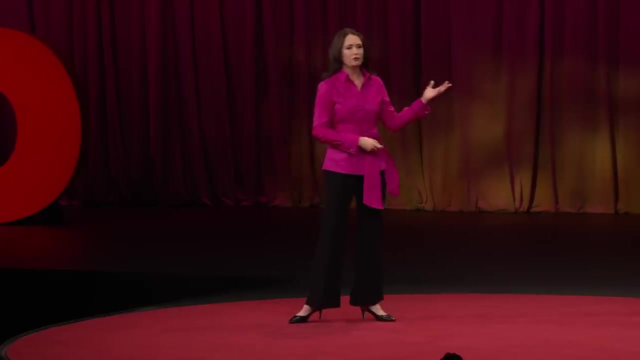 if we aren't proactive to shape the world we want. And what kind of world would we want? Well, in a resilient world, we compete to attract talent from across the globe and set the standard And set aside our nationalist tendencies. A shrinking world is in our future. but obviously some places are much closer than others. In the Democratic Republic of the Congo, Ethiopia, Nigeria, Tanzania, fertility is still high enough that each generation is twice the size of the one before it. Those young and growing populations can be a tremendous resource for their national economies. 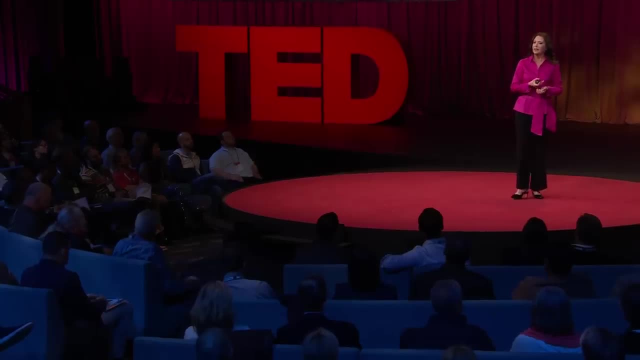 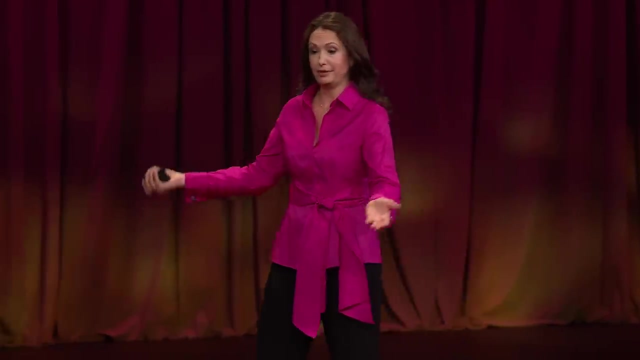 if we have investments in human capital and other policies that can help these countries reap a demographic And they can be a resource for the global economy too. I mean the US and Canada. they stand out as still growing, despite below-replacement fertility in both. And in fact, Canada had record population growth last year, 96 percent of which was due to immigration. Theirs aren't the only models for immigration, and there are obvious tradeoffs to opening your borders, But no one said this would be easy. 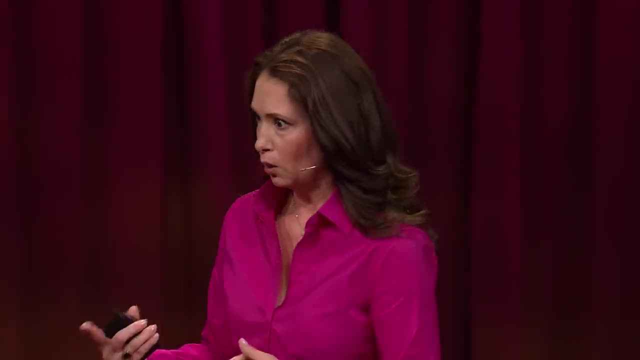 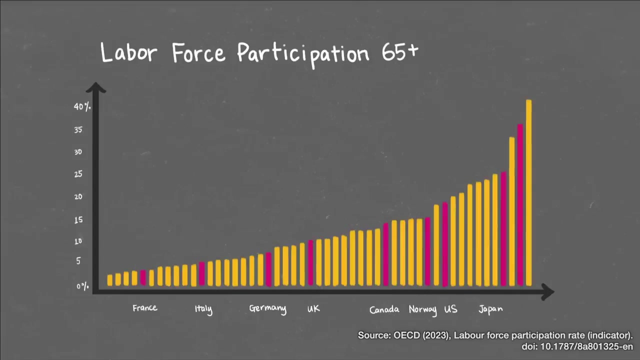 And speaking of things not being easy, we're going to have to work longer- Me too, You too- And that's because, in nearly half of the economies that the OECD tracks, fewer than 10 percent of people over the age of 65 still work. 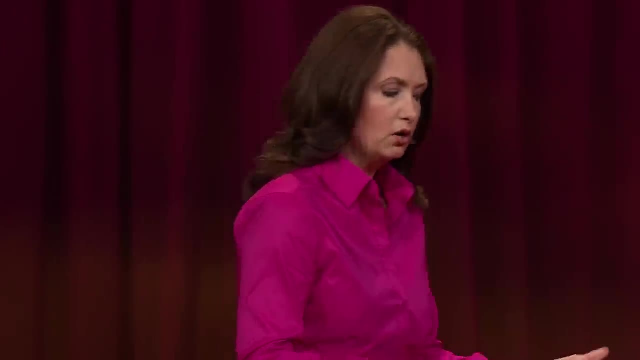 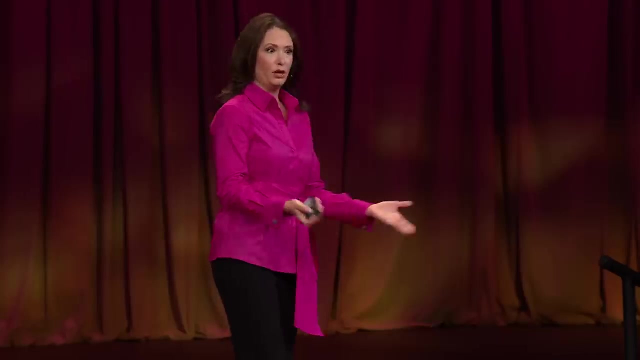 That is not going to fly in a resilient world. But in a resilient world we've rethought what work looks like at older ages and we strategically leverage technology to maximize our productivity And we can work longer because we're healthier. In a resilient world, we finally realize that investing in health 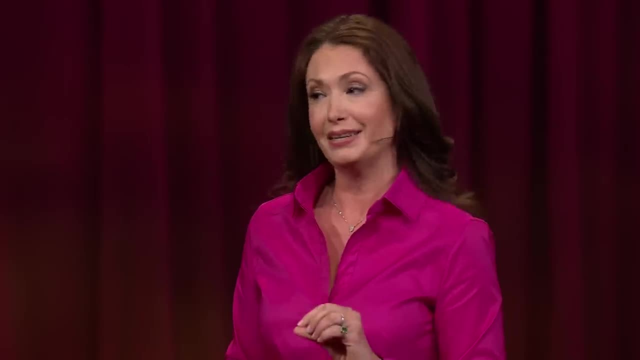 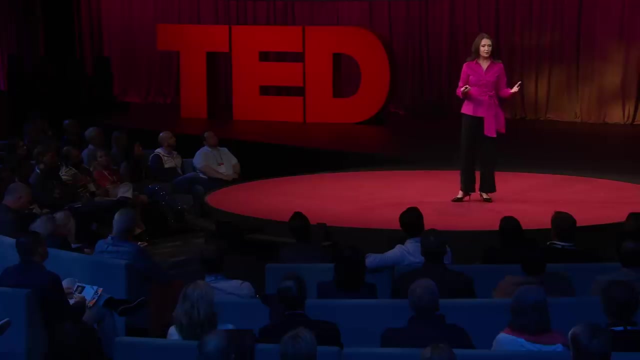 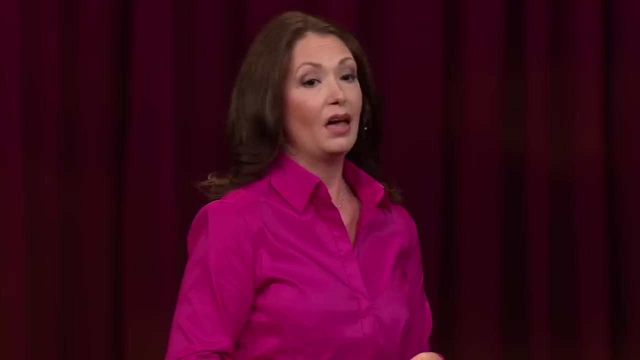 is a much better use of time and resources than trying to dictate population size. Similarly, in a resilient world, we've put in place policies, incentives and technologies that recognize how we consume is just as important as how many of us consume, and the environment is healing. 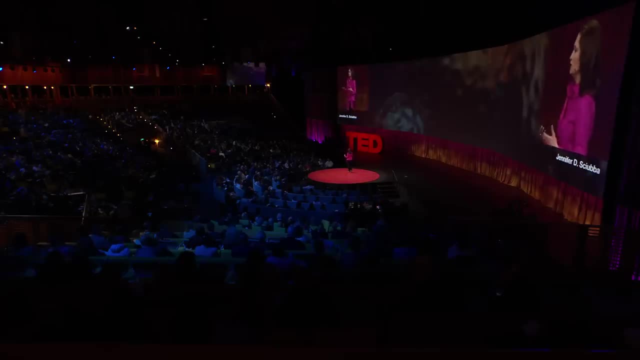 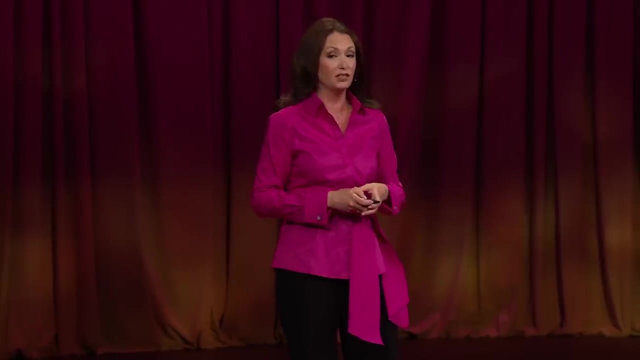 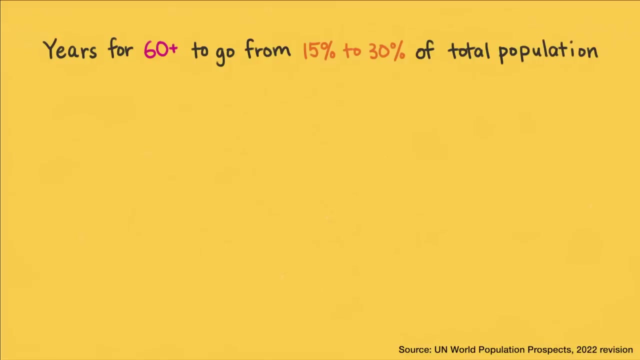 In a resilient world. those societies closer to the start of this demographic transition take advantage of the time to plan and institute sustainable, sustainable systems in the face of their demographic change. This is important because for the population ages 60 plus to go from 15 percent of the total to 30 percent,